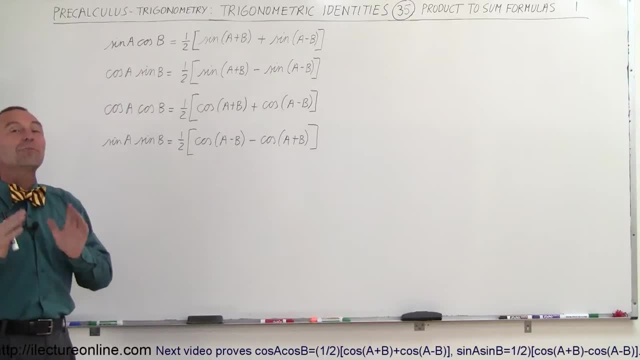 these. I've never been able to. I think I might have been able to for a few minutes, but an hour or two later I messed things up again. It's almost impossible to remember these four equations, So what I'm going to show you now is how to. 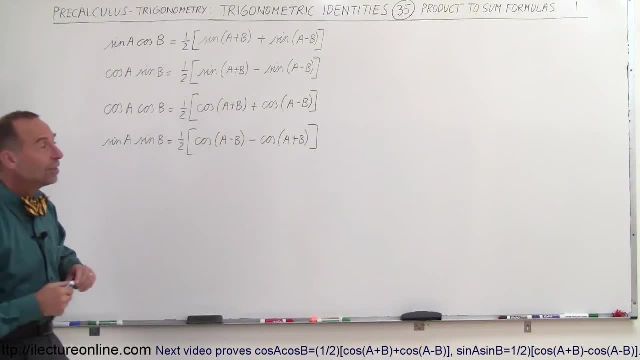 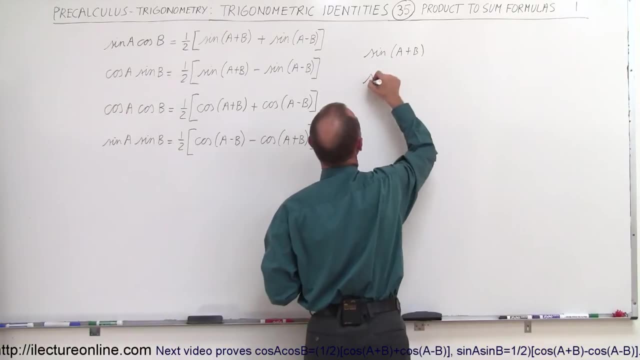 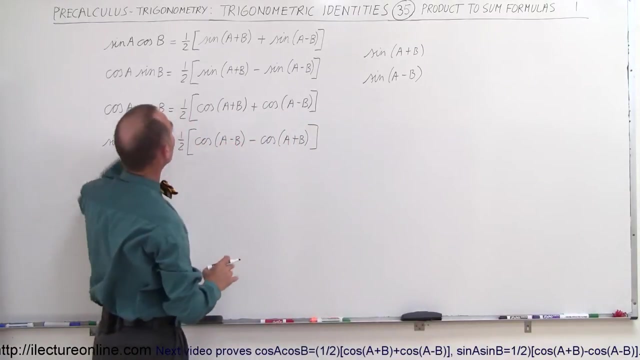 simply derive them fairly readily, and you do that by using these, By using the sine of A plus B and the sine of A minus B equation For the first two. So we'll start with the first one on top. How do we derive a? 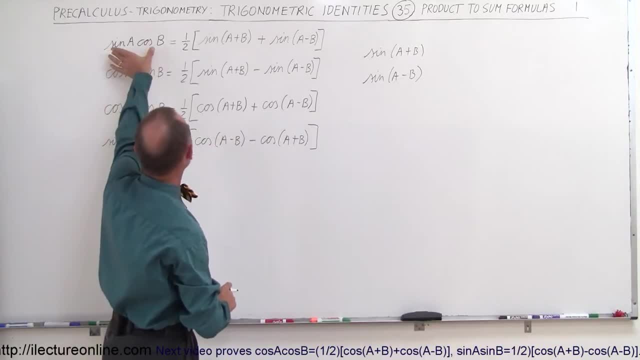 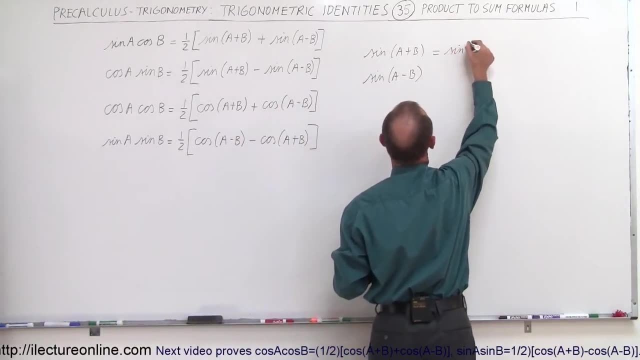 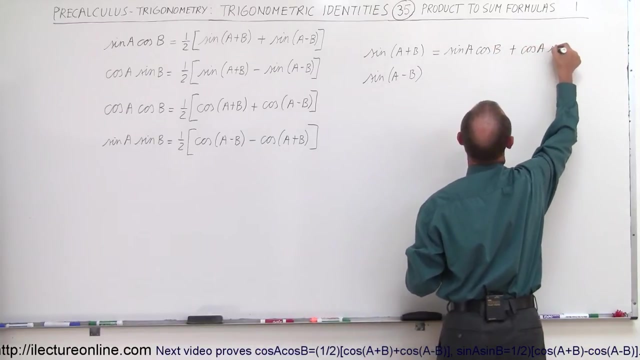 transformation or an identity that gets you from a product to a sum. Alright, so what are these equal to? The sine of A plus B is equal to the sine A times the cosine B, and if this is a plus, this becomes a plus plus cosine A sine B. and. 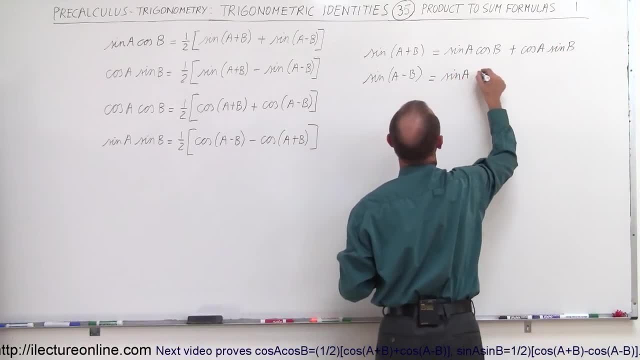 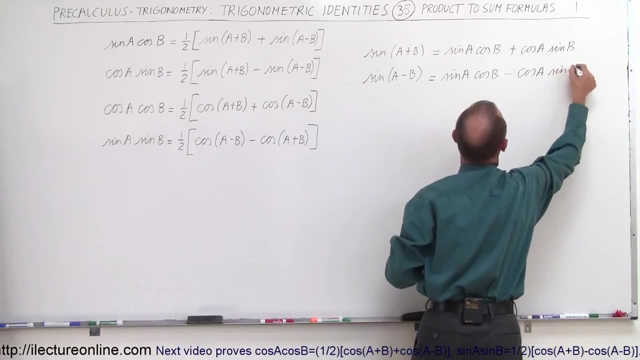 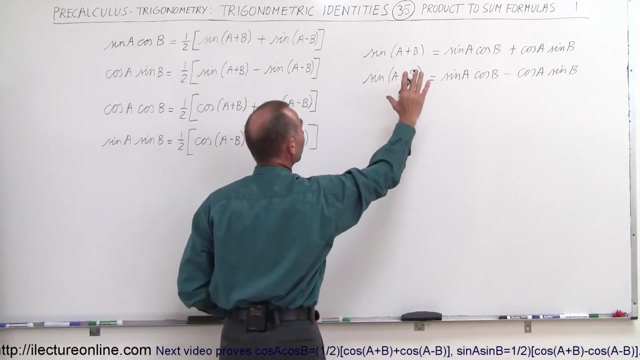 here. this one becomes the sine A, cosine B, and if this is a plus, this becomes a minus, this becomes a minus, and that would be cosine A sine B. So those are a lot easier to memorize than these right here and it's simply, it's very fairly. 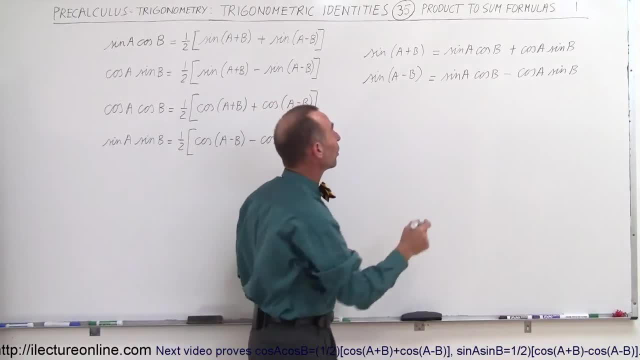 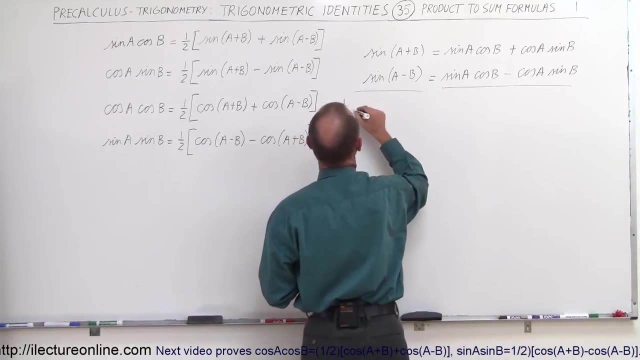 simple to go from there to there. so that this is how you do that: Let's add both sides together. So we're going to add this side and we're going to add the right side together, and what we get? so we get the sine of A plus B plus the. 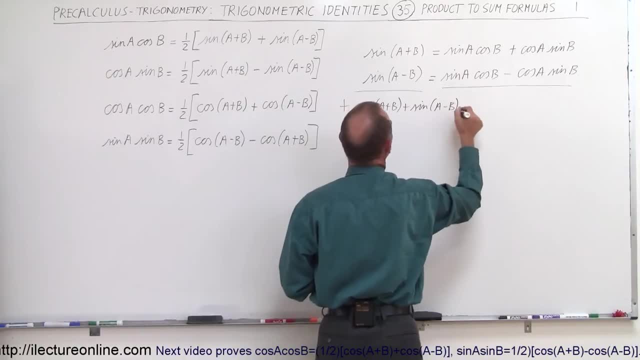 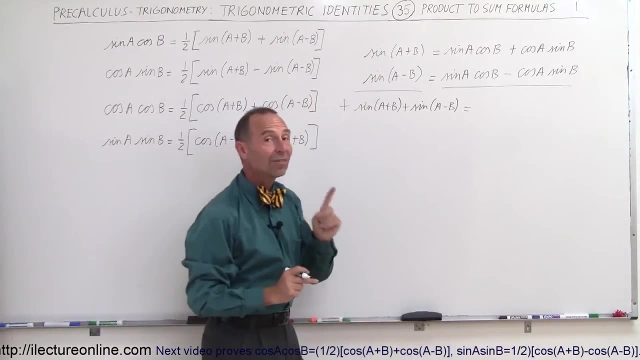 sine of A minus B. minus b is equal to: and now notice that we have the sine of a plus b and the sine of a minus b, which is what we have right there. And now let's see what happens when we add the right side. 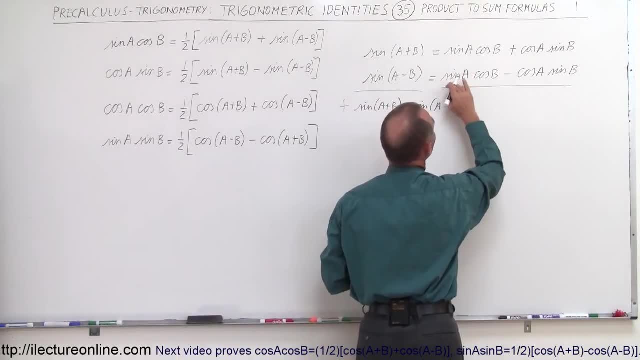 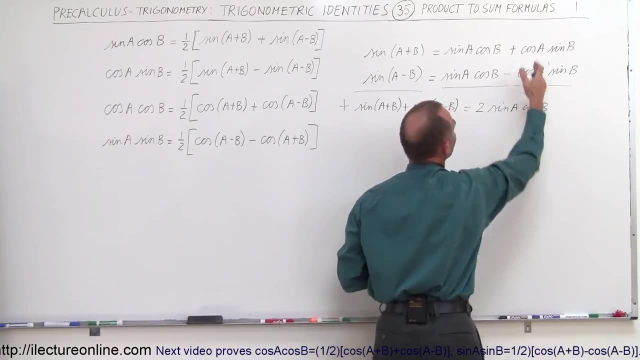 together. Well, we have the sine of a cosine of b and the sine a cosine of b. So when we add those together we get two times the sine a times the cosine b. And if we add these two together, notice this is a cosine a sine b, cosine a sine b. When we add them together we get zero. 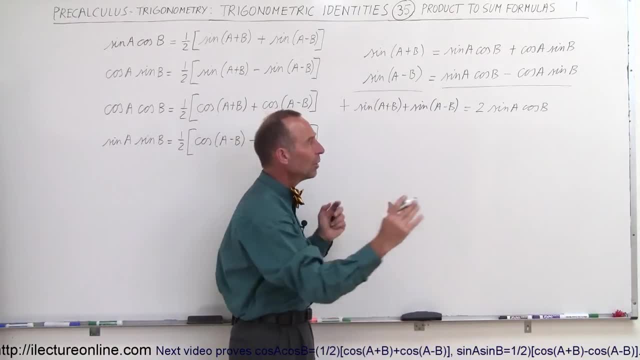 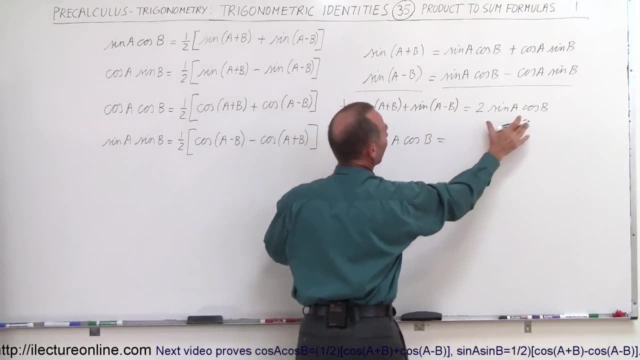 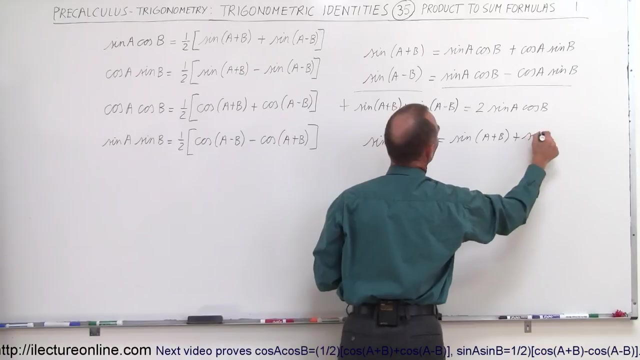 so we end up with this and then if we divide both sides by 2 and turn the equation around, we now get the sine of a times the cosine of b is equal to. so we take this is equal to the left side, which is the sine of a plus b plus the sine of a minus b, and then we divide both sides of the. 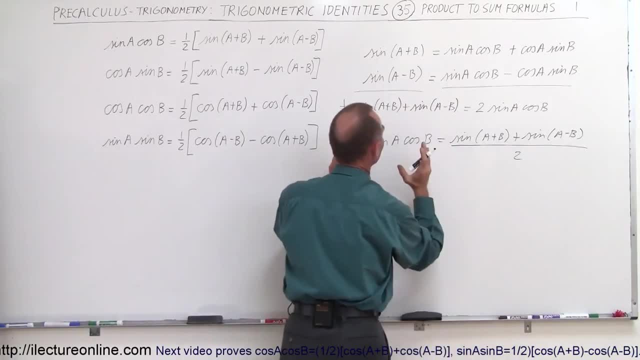 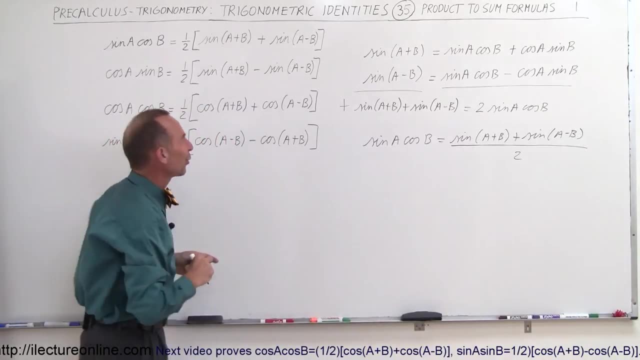 equation by 2. divide this by 2 and notice that now we get exactly what we have right on top there. so that is the easy way to quote, memorize those four equations. I much rather do that than do this, because I can never hang on to which is which and which is positive, which is negative in these. 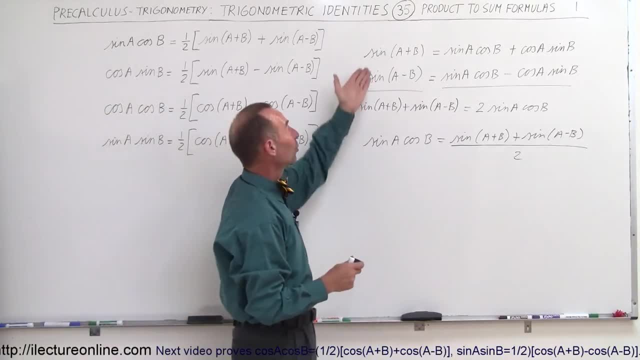 relationships, but that makes it a lot easier. then all you have to remember is what the sine of a plus b is, the sine of a minus b, and then later you'll see. you have to remember what the cosine of a plus b and the cosine of a minus b is equal to, and then you can easily derive these four. 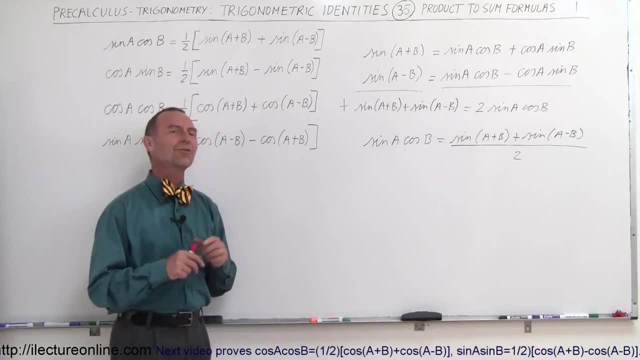 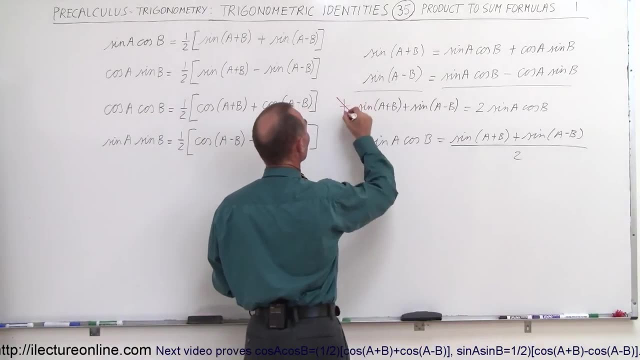 equations. so here's the first one, if you want. all right, I thought I'd just quickly show you how to get the second equation. we do exactly the same thing as we did before, but instead of adding them, we're going to subtract the two from one, from one another. so if we do that, subtract this from that or this from that. I should. 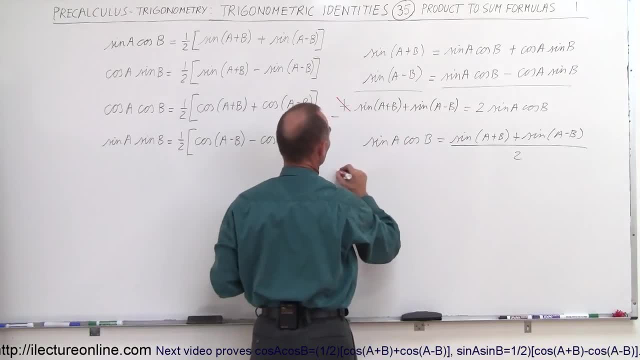 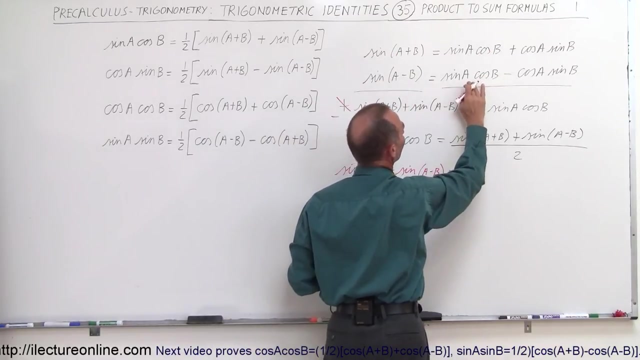 say, because we have sine of a plus b minus, sine of a minus b, so end up at the sine of a plus b minus, the sine of a minus b. of course, if I subtract this from that, I need to subtract this from that. so if I subtract this from that, I get zero. 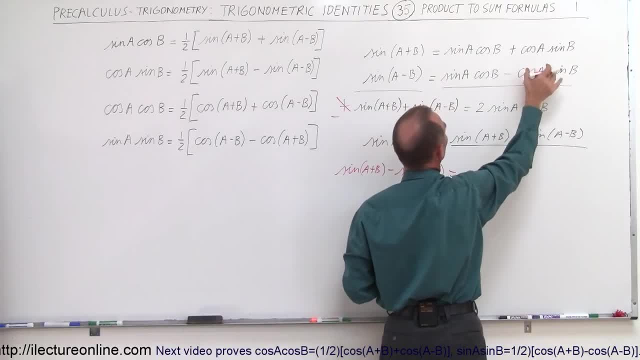 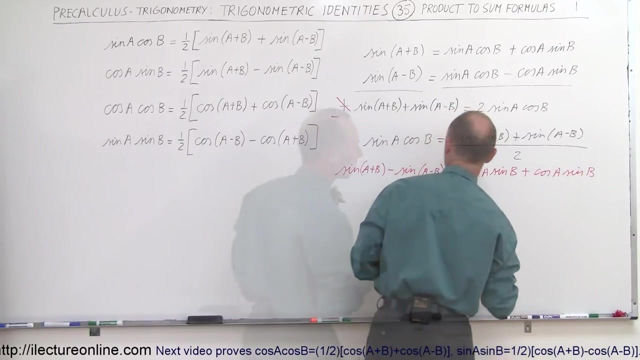 subtract and then, of course, i'm going to subtract this from that. if i subtract this, this becomes a positive. so end up with the cosine of a times the sine of b. minus a minus becomes plus the cosine of a times the sine of b and, of course, if you see, that's exactly the same. so i have two of them. 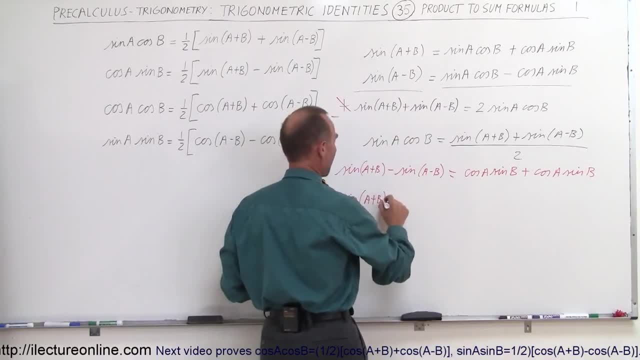 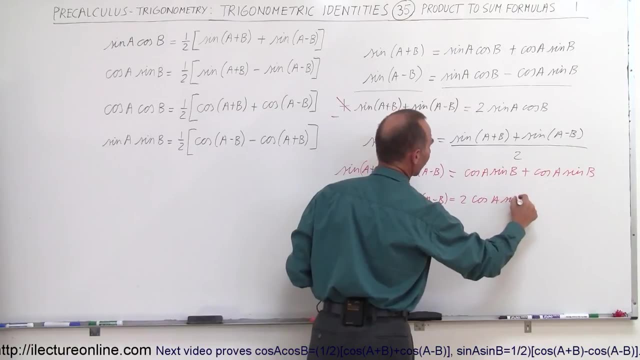 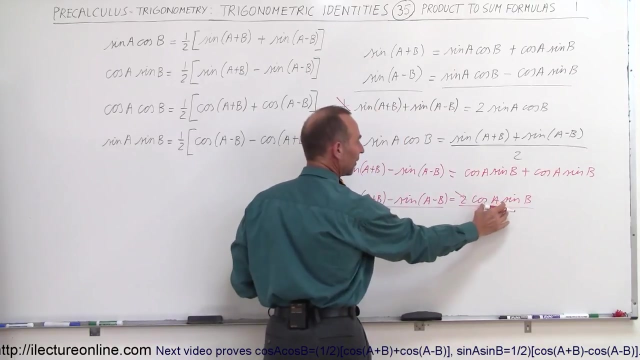 right now. so i can say that the sine of a plus b minus the sine of a minus b is equal to two times the cosine of a times the sine of b, and then if i divide both sides by two, this cancels out, and now i have the cosine of a times the sine of b is equal to this, which is exactly the same as the second. 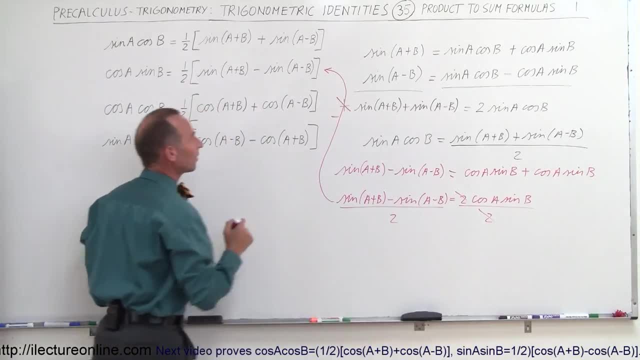 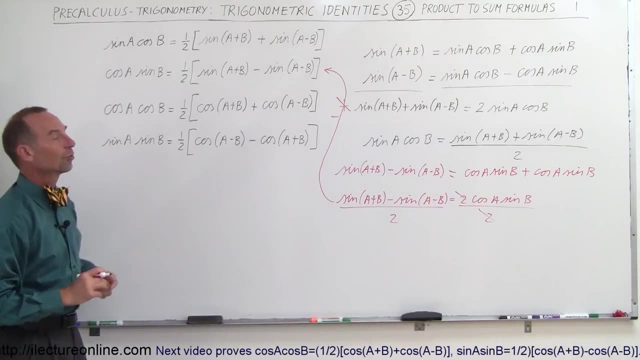 equation like that and that's how we can show you how we derive the first two product to sum conversions. and so, if you're interested in this, i'll, in the next video, i'll show you how to do the next two you.